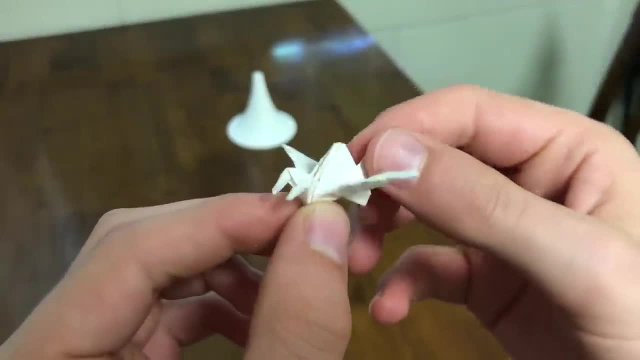 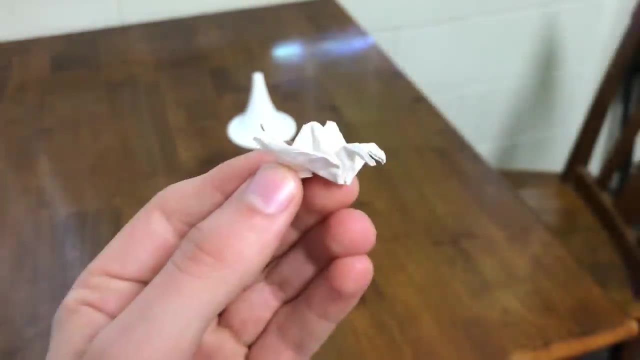 And while you do, I'll introduce you to one of his friends. This guy does have a tail and he also has two heads. This gives him five appendages: two heads, two wings and one tail, which means that he's made out of a pentagon. 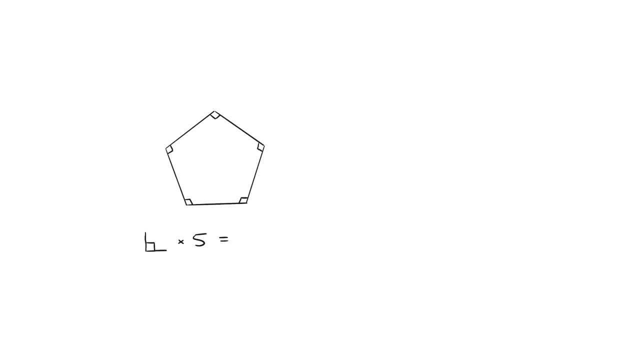 And, like his friend with no tail, if we look at each one of his corners, they all end in a 90 degree angle, which means that he has 450 degrees total. That's not enough to be a pentagon, So unless I'm tricking you with extra paper or something, 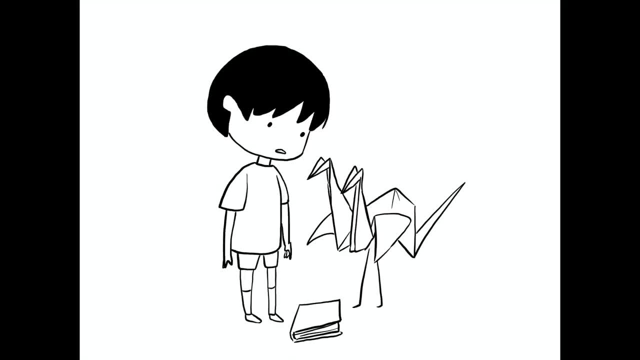 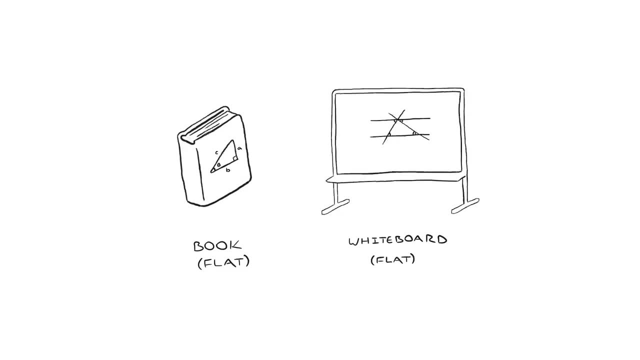 these two cranes break all the rules of geometry that you learned in school. So here's the thing: When you learned geometry, you learned it from books and whiteboards, where this stuff is true, But our cranes are not made from flat pieces of paper. 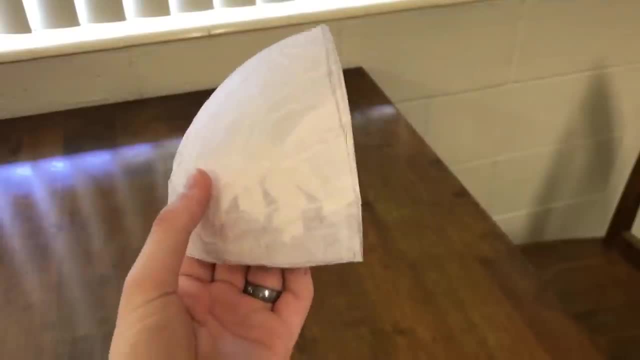 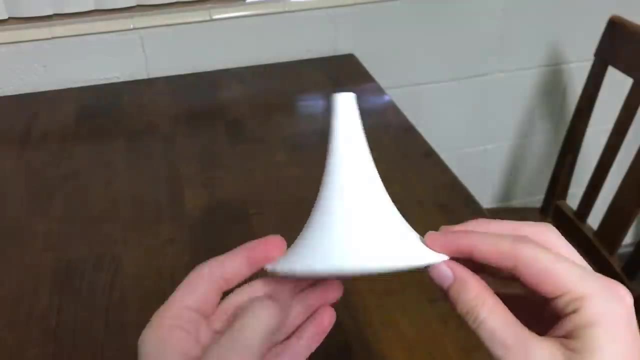 Our no-tailed crane is made from a sphere, a triangle cut from a sphere, And our, Our two-headed crane is made from a pentagon cut from a shape called a pseudo-sphere On a sphere, every triangle adds up to more than 180 degrees. 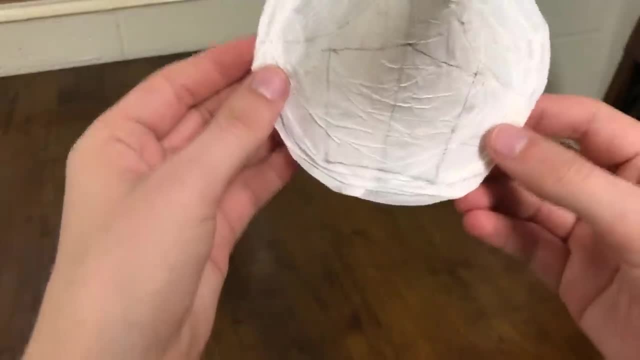 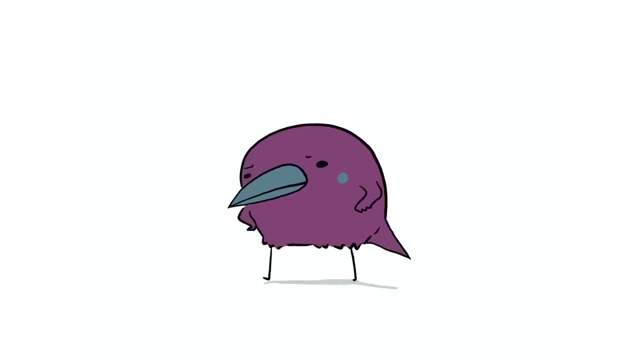 And on a pseudo-sphere, every triangle adds up to less than 180 degrees. Now I know what you're thinking. That's cheating. The edges of those triangles aren't even straight lines. Flat geometry is the normal geometry. It's the one that we live in. 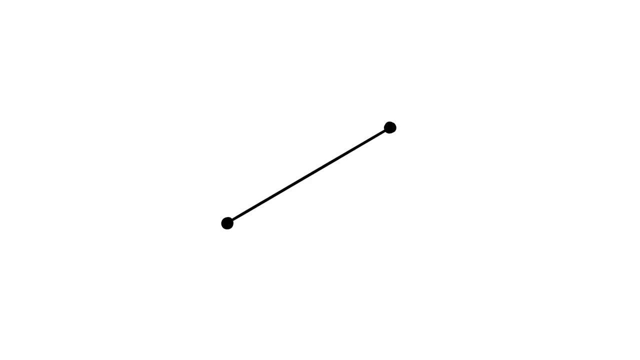 Yeah, says who. A line is the shortest path between two points And if you're confined to the two-dimensional surface of a sphere, then a straight line is always a segment of a circle. Yeah, in three dimensions we could imagine cutting through. 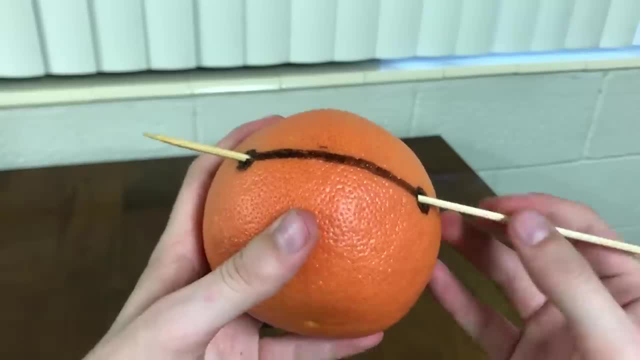 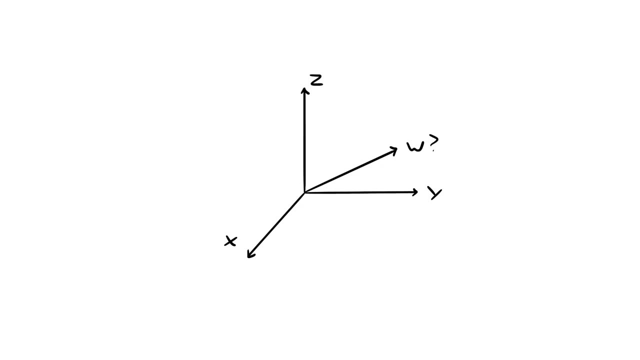 digging a hole through Earth to make an even shorter path. But if you live in two dimensions, that's all you have. As three-dimensional creatures we can't travel or even imagine a fourth dimension. The three dimensions is all we have. So if our three-dimensional space is curved, 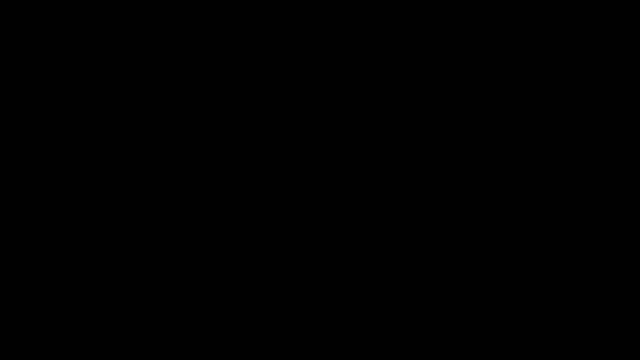 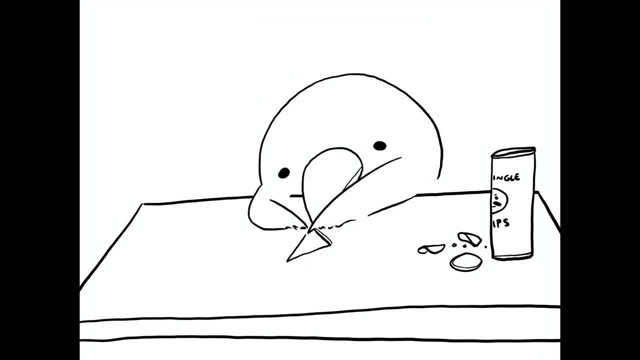 our straight lines might not be that straight at all. We could live in a universe where triangles don't add up to 180 degrees, but we just don't realize it because we're so small. So in this video we're going to use the rules of origami. 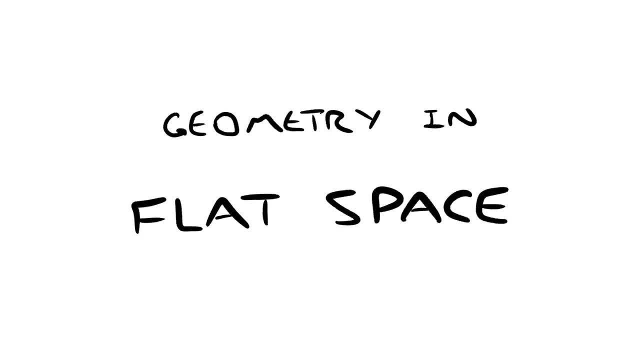 to figure out the shape of our universe. The way that we learned geometry in school has stayed pretty much the same since about 300 BC. This is when the Greek mathematician Euclid wrote his treatise Elements. In the first book of Elements, Euclid gives five axioms of geometry. 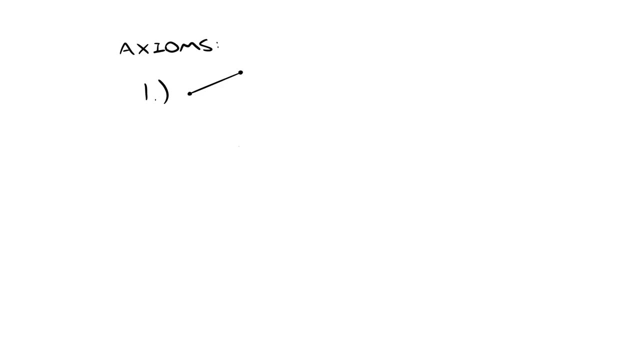 And from these you can prove any other fact. They are: one: you can draw a straight line between two points. Two: a line segment can be extended infinitely. Three: if you have a center and a radius, then you can draw a circle. 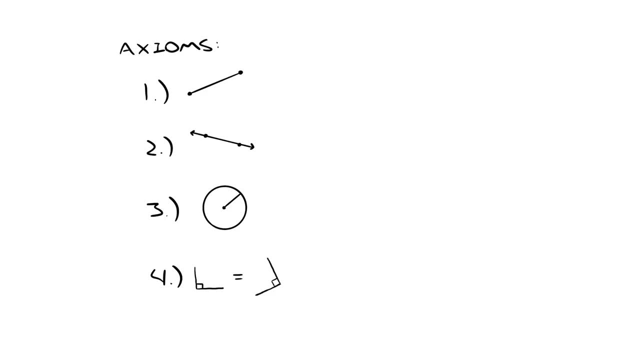 Four: all right angles are equal to each other. And the fifth one say you have two lines and a third line that intersects both of them. If the interior angles add up to less than two right angles, then the two lines will always intersect each other. 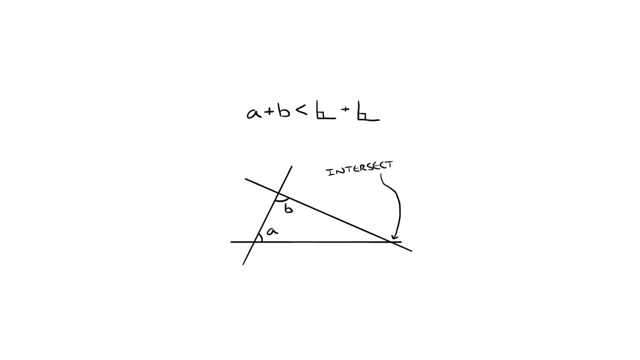 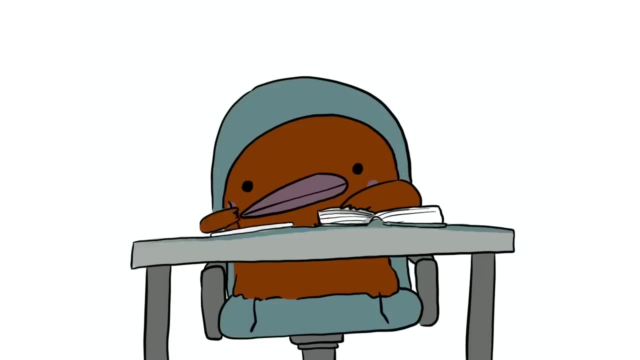 Now, ever since Euclid wrote these down, mathematicians have had a problem with this fifth one because it's ugly, It's long and it's confusing. It sounds so arbitrary that they thought maybe they could prove it from the other four to get rid of it. 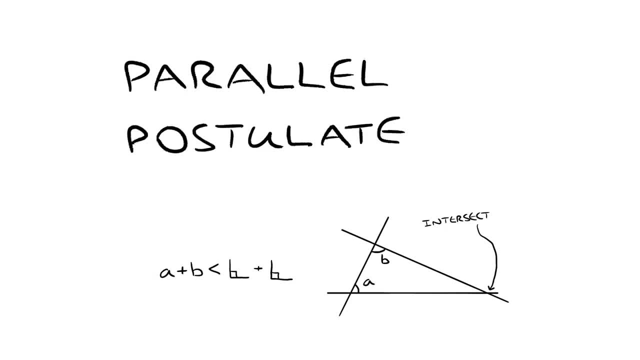 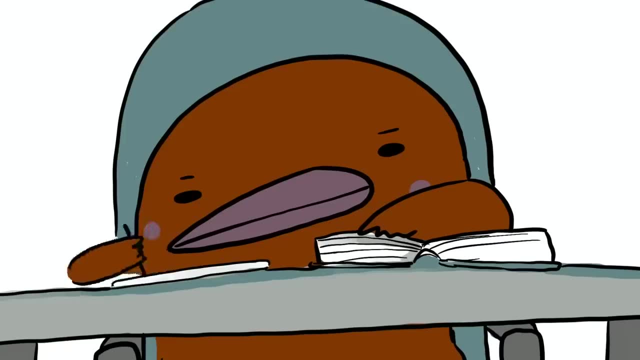 We now call the fifth axiom the parallel postulate, And trying to get rid of this thing became the focus of mathematicians all over the world, But all they could ever do is replace it. They would come up with different axioms, but there would still be five of them. 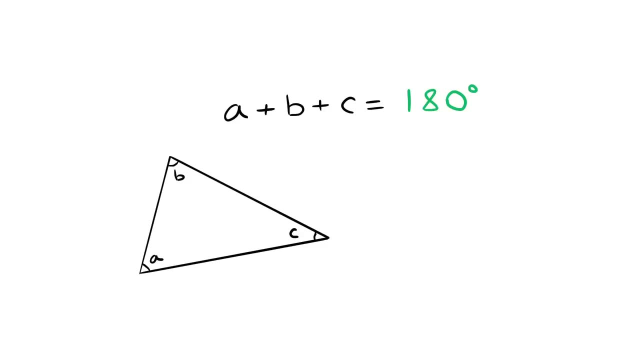 You already know one of these replacement axioms because it's how we started off the video. today, The angles in a triangle add up to 180 degrees. This is the same thing as the parallel postulate. Let's draw two lines that never intersect, also known as parallel. 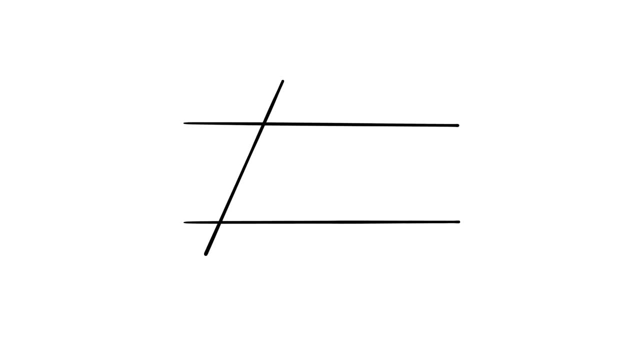 Now let's draw a third line that goes through both of them. According to Euclid's fifth, these two angles must be 180 degrees. If there were any more, then the two lines would intersect on the left. If there were any less, the two lines would intersect on the right. 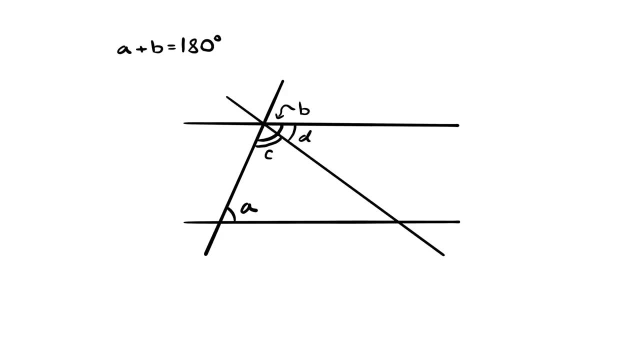 Now let's draw a fourth line that splits B into two angles. Clearly, B equals C plus D, and this angle here must be the same as D. You can now see that we've made a triangle between A, C and D, And if we plug in we get A plus C plus D equals 180 degrees. 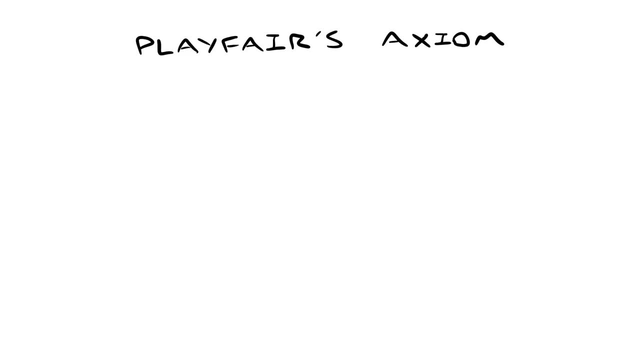 Another replacement that mathematicians found is called Playfair's axiom. It says that if you have a line R and a point P that's not on R, then there's only one line that you can draw through: P that doesn't intersect R. This, of course, is the line that's parallel to R. 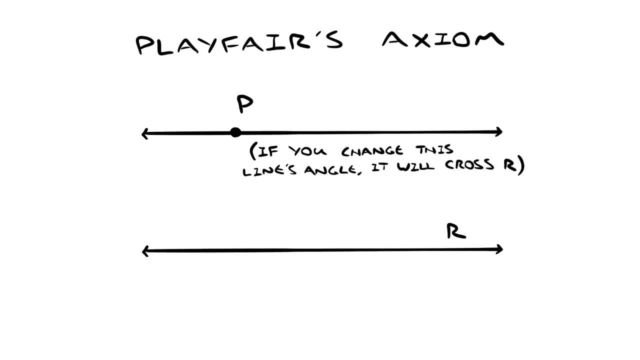 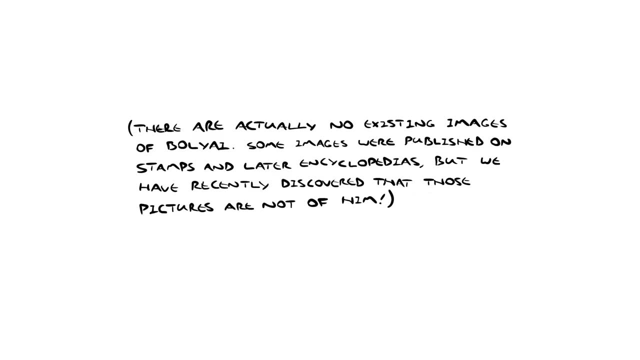 You can probably see how that's related to the parallel postulate, so I'll leave it up to you to prove. So in 1820, Hungarian mathematician Janos Bolyai was studying the parallel postulate, specifically in the form of Playfair's axiom. 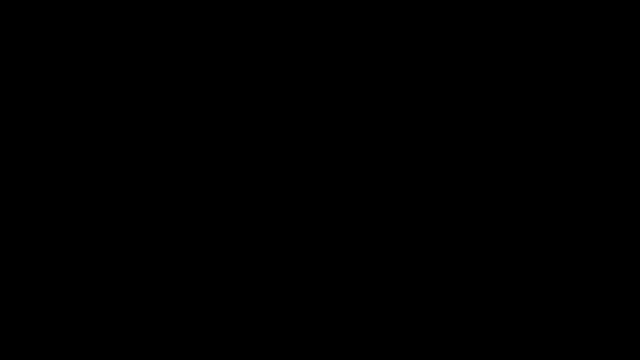 His father, Farkas, was also an accomplished mathematician and he thought it was a waste of time. He told Janos that the topic extinguished all light and joy in his life. A little bit dramatic, but Janos continued to study it. 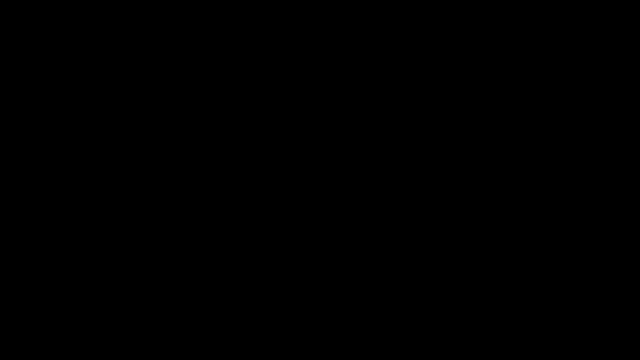 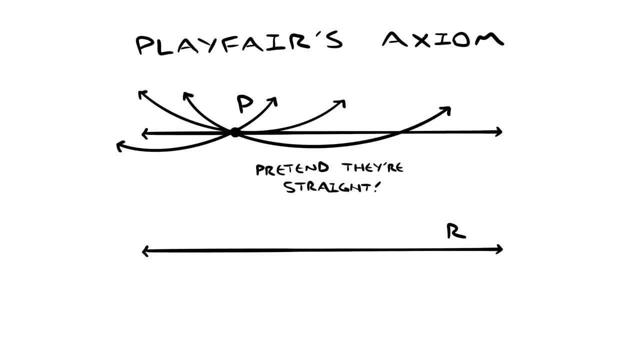 Bolyai started by assuming the opposite of Playfair's axiom. He said: let's pretend that if you have a line R and a point P not on R, then you can always draw more than one line through P that never crosses R. 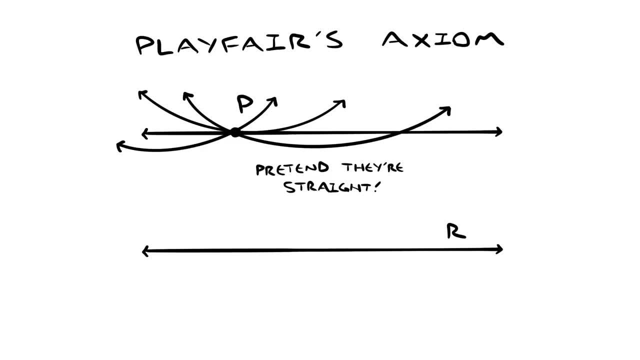 This might have been a good way to start a proof by contradiction, but there was never a contradiction. Bolyai discovered all these new properties that geometry would have if this were true, and they were different from Euclid's geometry, but they all made sense. they were logically sound. 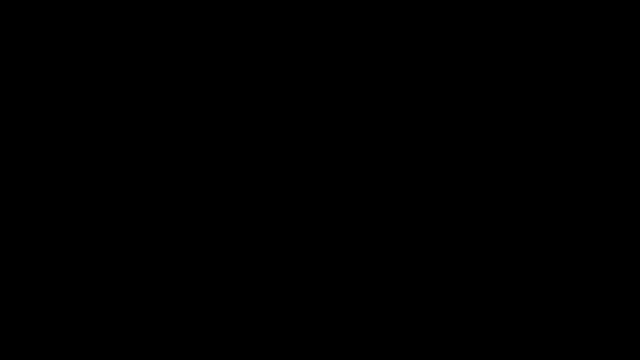 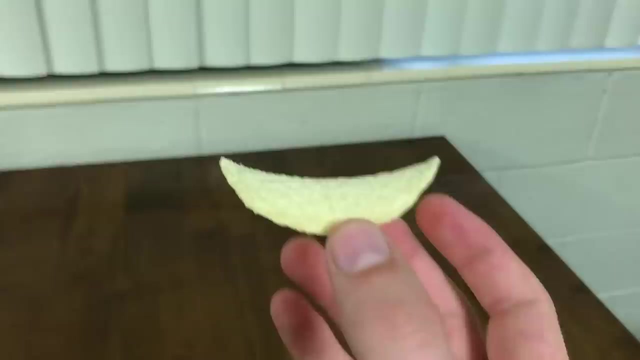 The only problem was that he couldn't draw it, at least not on paper, But he could have drawn it on this. The shape of this pringle can be approximated by a hyperbolic paraboloid. The cross-section is an upward parabola in one direction and a downward parabola in the other. 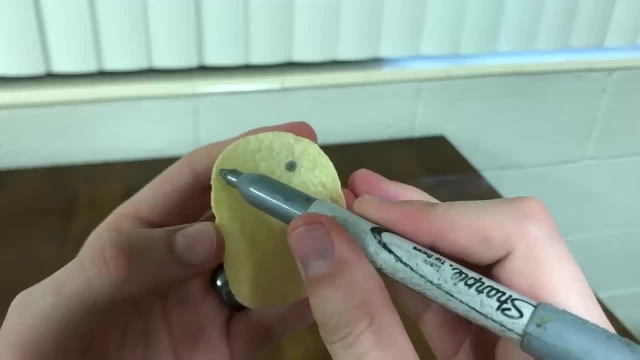 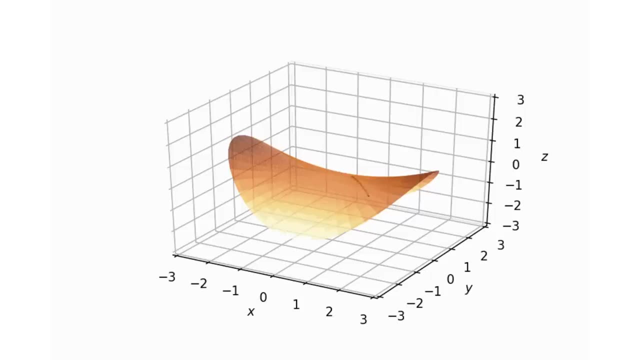 One of the interesting properties of this shape is that the shortest path between two points bends outward, away from the center. So if we try out Playfair's axiom, we draw a line R down the center and then we draw a point P above it. 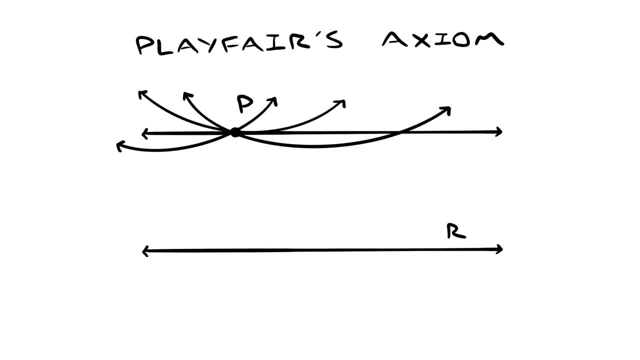 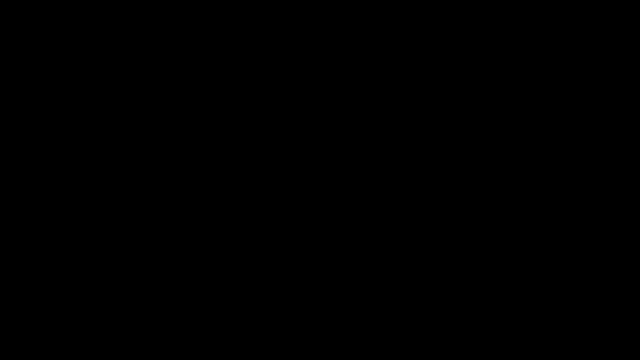 then we can draw as many lines through P as we want. Euclidean geometry is not true on this potato chip, but Bolyai's is. It's pretty weird that it took us this long to discover alternatives to Euclidean geometry, because we're literally living on one. 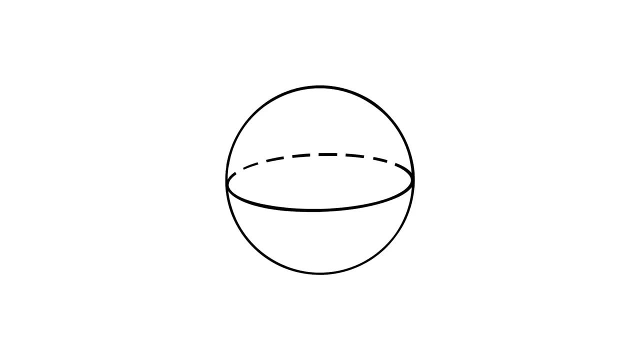 Try out Playfair's axiom on a globe, Of course, keeping in mind that straight lines are great circles, like the equator or like longitude lines, but not like latitude lines. So draw a line R and a point P, and what you'll notice is that every line that you can draw is going to cross through R. 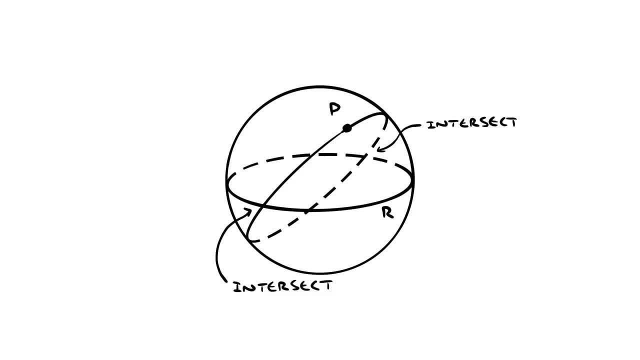 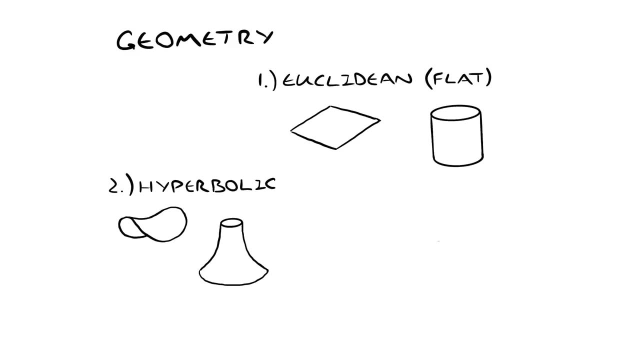 There's no such thing as a parallel line on a sphere. Now we've discovered three types of geometry. One is flat, Euclidean geometry. Two is the one that Bolyai discovered, which we now call hyperbolic geometry. It takes place on surfaces with negative curvature. 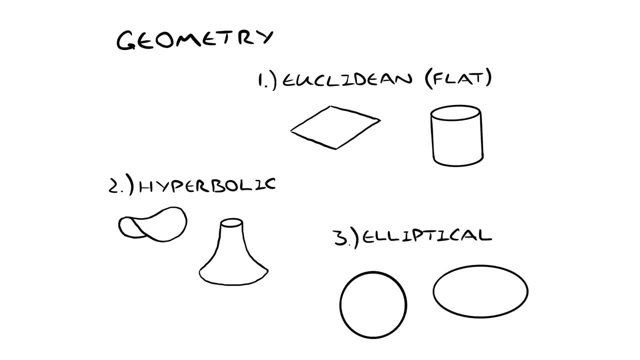 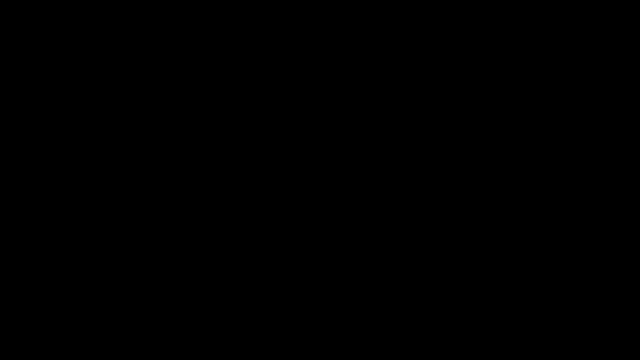 And then the third is elliptical spherical geometry, and it takes place on surfaces with positive curvature. So far, all the examples I've given you have been in 2D, because that's all we can visualize. A sphere is a 3D object, but the surface itself is two-dimensional. 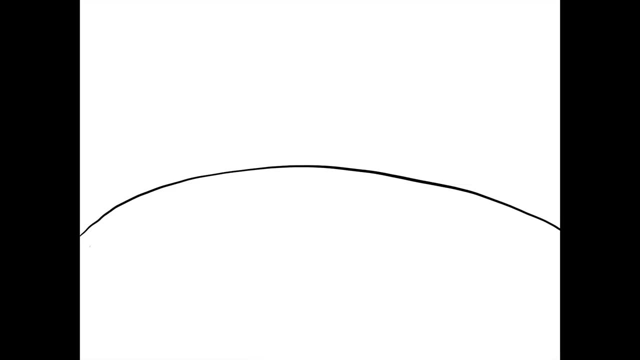 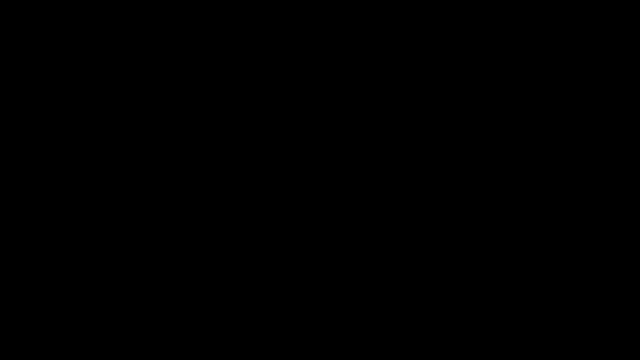 A 2D creature could live on the surface of the sphere, but they would never be able to imagine the sphere itself. Similarly, we can't imagine curved 3D space, But it is possible, and Bolyai realized this At the end of his book. he wrote that we need to do experiments to figure out whether our universe is curved or flat. 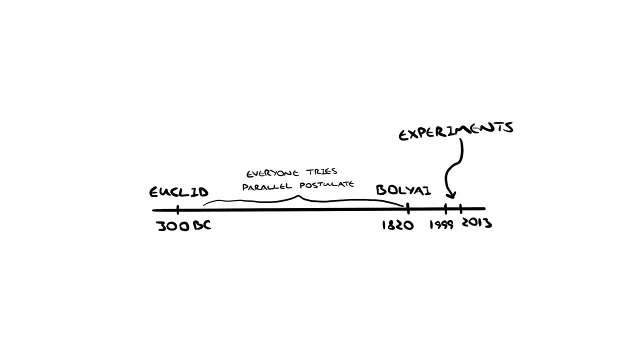 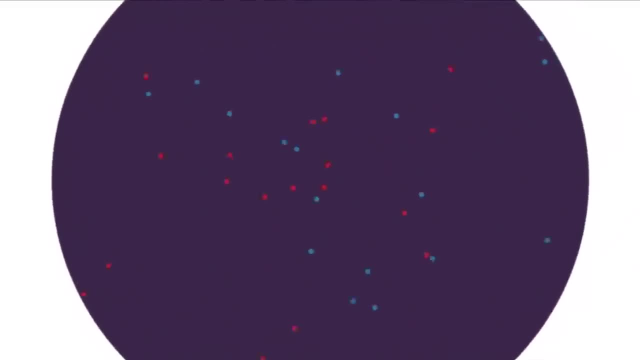 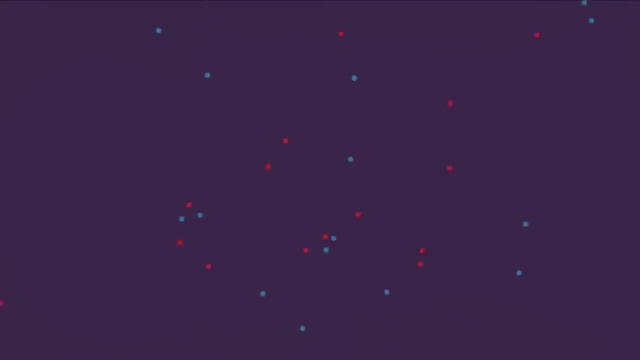 Between 1999 and 2013,. we got the evidence we needed to figure this out. Immediately after the Big Bang, the universe was a hot, dense fluid of elementary particles. As it expanded, it got less dense and since wavelengths increased, it got less energetic too, and it cooled down. 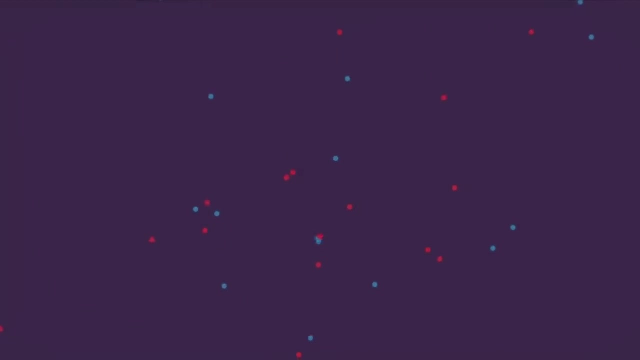 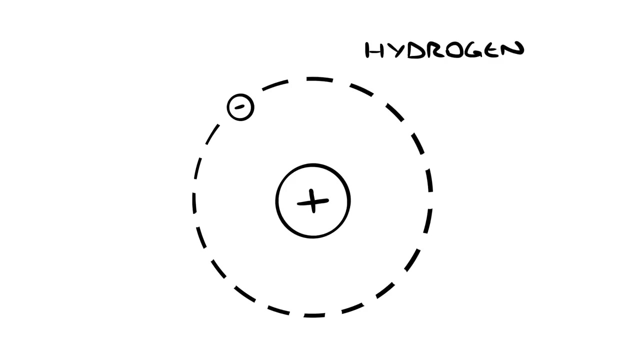 When the universe was about 370,000 years old, particles had cooled enough that electrons could become bound to protons to form hydrogen. This is the first time the universe had atoms. When electrons and protons combine to form hydrogen, it releases light at a specific wavelength. 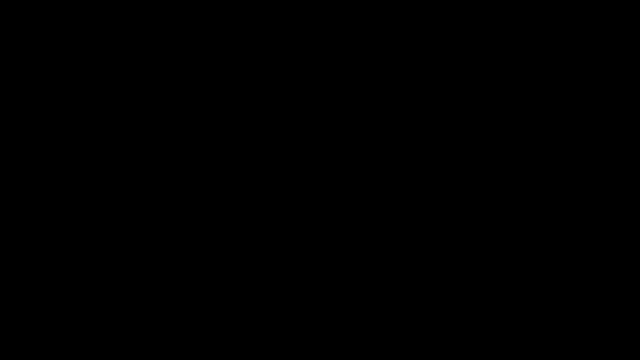 This light is still around today, but because the universe has been expanding, it's been redshifted to the microwave spectrum. If you point a telescope anywhere in the sky, you'll see this leftover radiation, So we call it the cosmic microwave background. 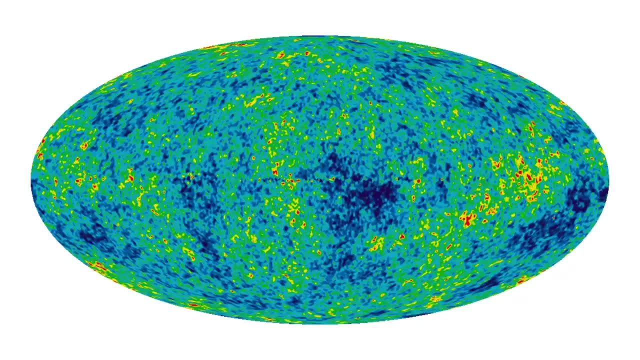 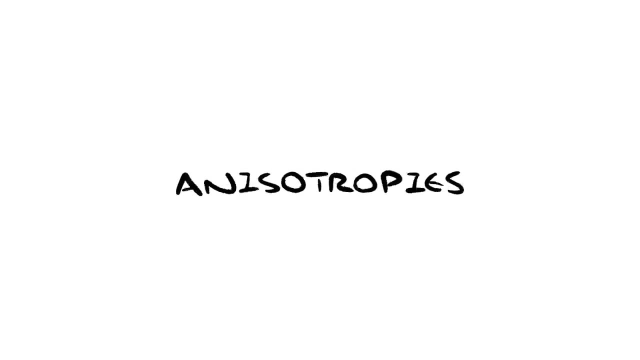 The temperature of the CMB is mostly uniform, but if you measure it really precisely there's tiny differences from one place in the sky to another. These are called anisotropies, and they teach us all kinds of things about our universe. 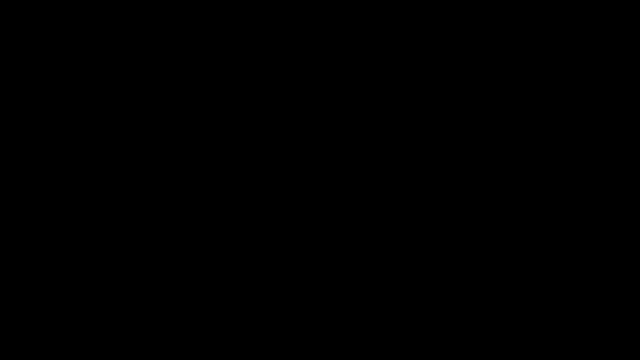 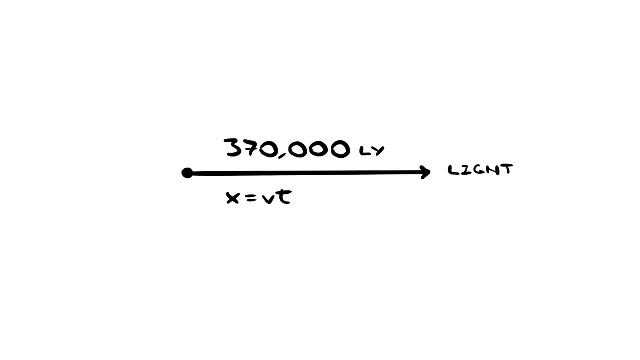 When the CMB formed, the universe was pretty young, but it was already a decent size. Remember it was about 370,000 years old, which means light could have traveled a maximum of 370,000 light years, But the universe was already bigger than 370,000 light years wide. 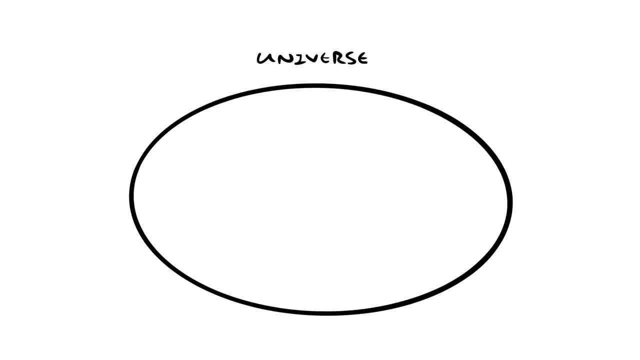 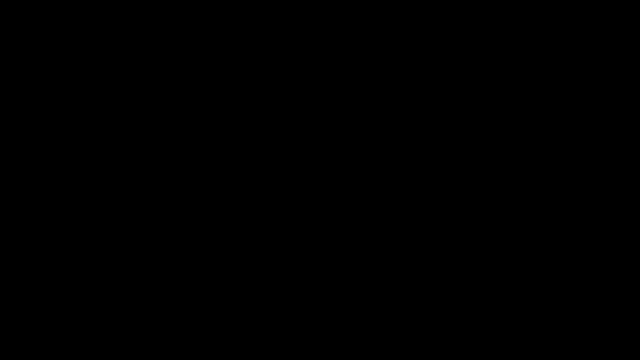 If a beam of light would have had the entire age of the universe to travel from one side to the other, it wouldn't have been able to make it. If light couldn't make it, then nothing could have made it, and that even includes the influences that transfer heat. 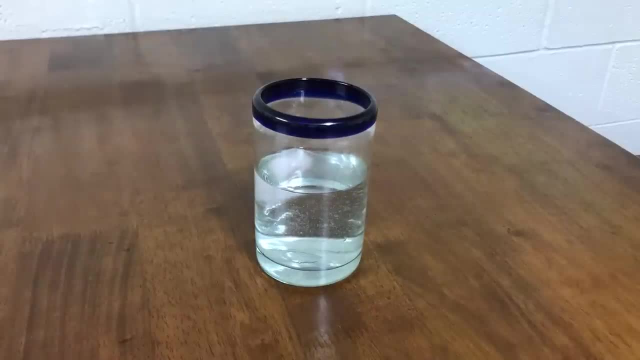 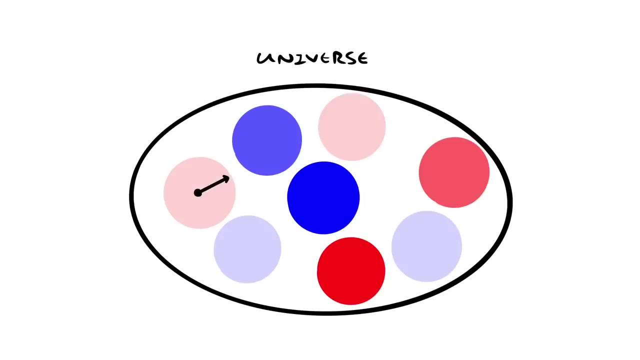 It takes a few minutes for ice to melt in a cup of water and for all the water molecules to reach the same temperature. Similarly, the universe wouldn't have had enough time to reach thermal equilibrium When the CMB formed. there were all these patches of slightly cooler and slightly hotter spots, and that's where these anisotropies come from. 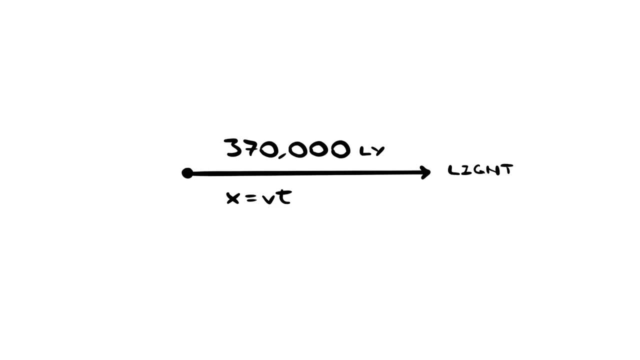 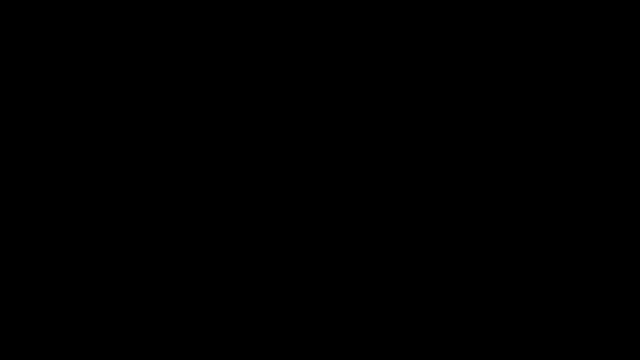 We know the speed of light and we know the age of the universe at that point, so we can figure out how big these patches should have been. We also know the size of the universe then and the size of the universe now, so we can use a little bit of trigonometry to figure out how big these patches should look in the sky. 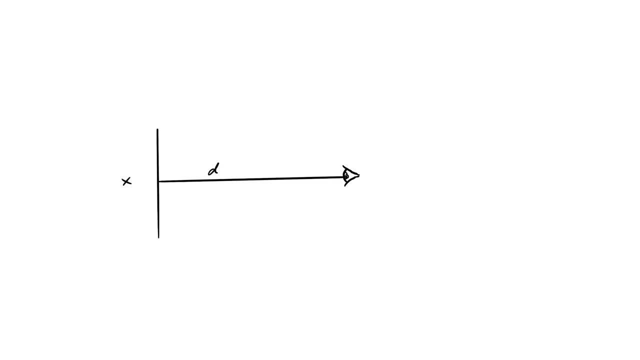 Say you're looking at an object of width x from a distance d away. You can draw a triangle between your eye and the two edges of the object and then you can split that into two right triangles. Now, tangent of theta over 2 equals opposite over hypotenuse. so x over 2d. 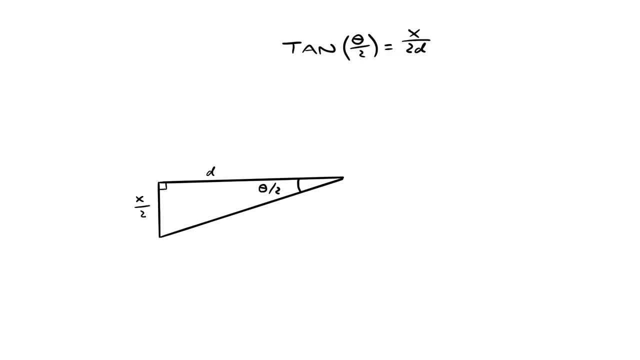 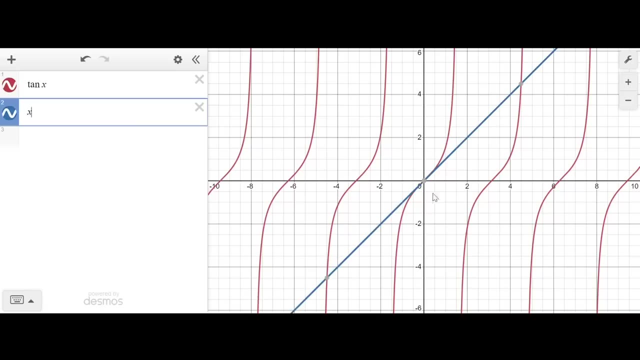 Now remember, this is space we're talking about, so d is huge and x is not as big, So it's not going to take up a very big angle in the sky. For small angles, tangent of a is approximately equal to a. 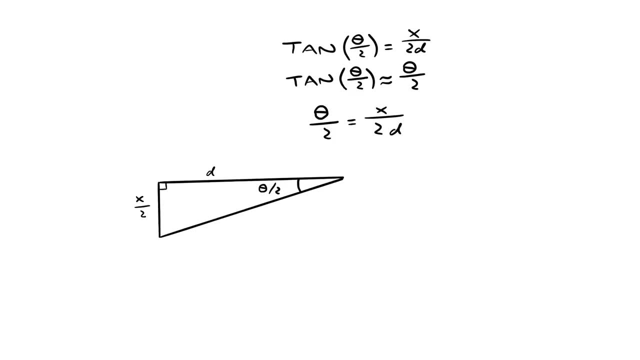 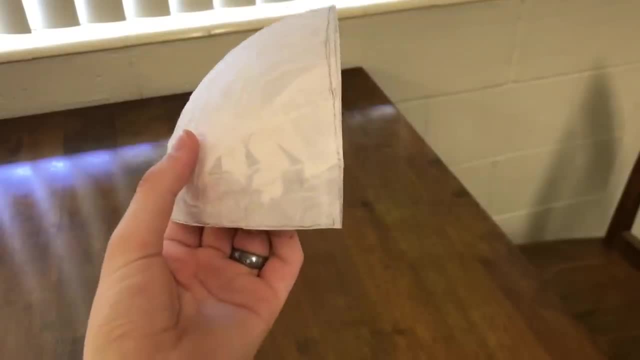 So we can safely say that theta over 2 equals x over 2d and therefore theta equals x over d. But what if we live on a big four-dimensional sphere? Remember, in elliptical space, triangles add up to more than 180 degrees. 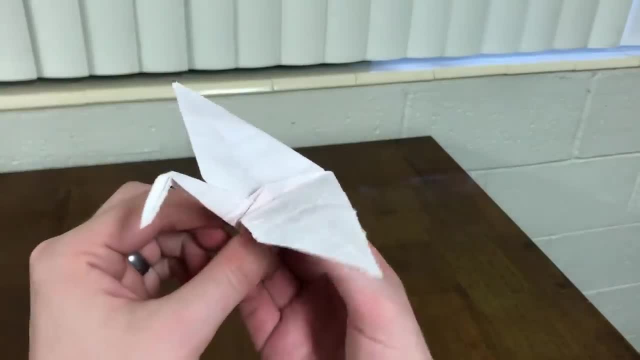 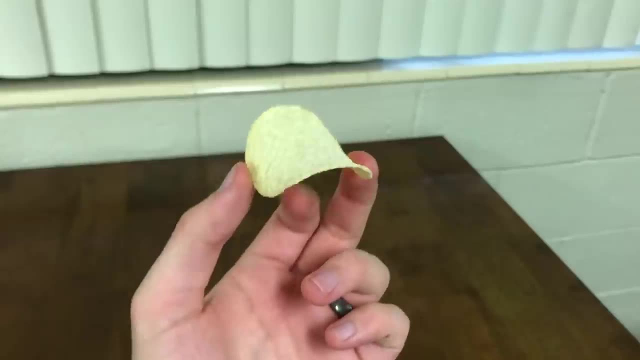 This is the same trick we use to make our no-tailed crane, So theta should be bigger than what we expect. What if we live on a big four-dimensional pringle? Well, we know, in hyperbolic space, triangles add up to less than 180 degrees. 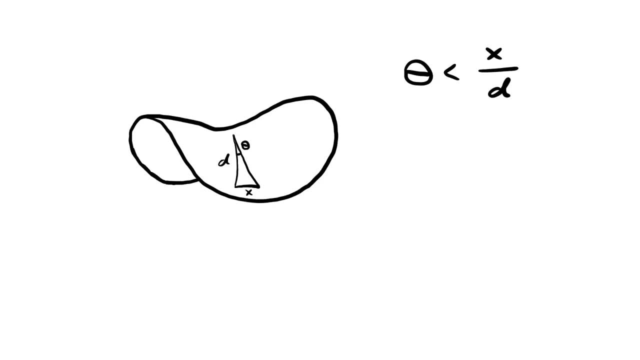 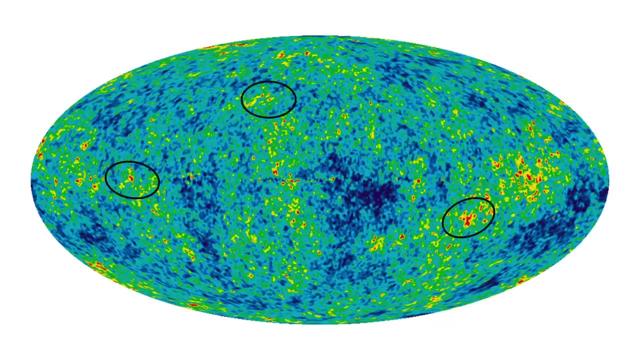 This is how we made our two-headed crane, So theta should be smaller than x over d, And that's it. All we need to do is measure the temperature of the CMB all over the sky. look at the size of these patches. 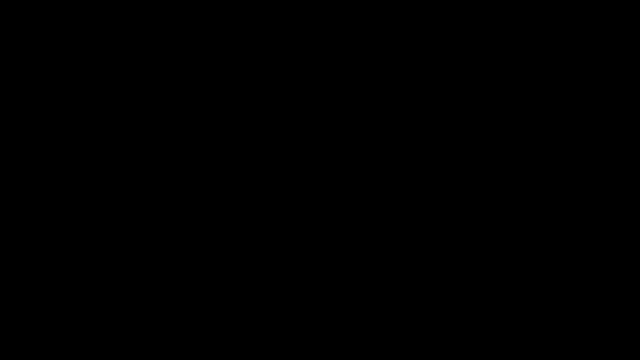 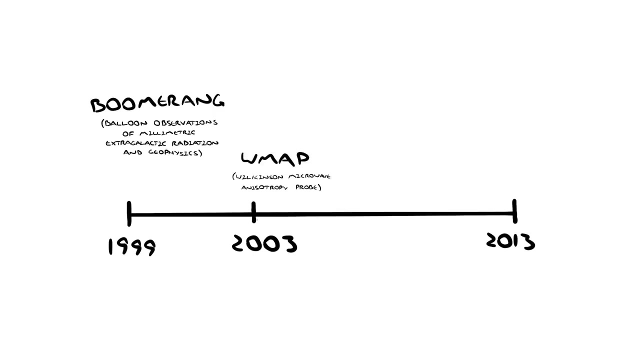 and that will tell us whether our universe is curved or flat. The CMB was first measured with a high enough resolution to do all this, in 1999 by the Boomerang experiment, and then again in 2003 by the Wilkinson Microwave Anisotropy Probe. 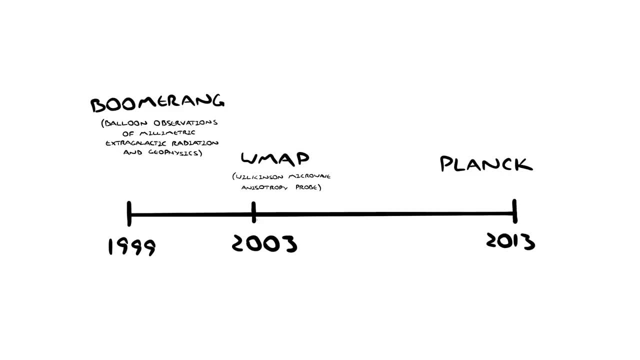 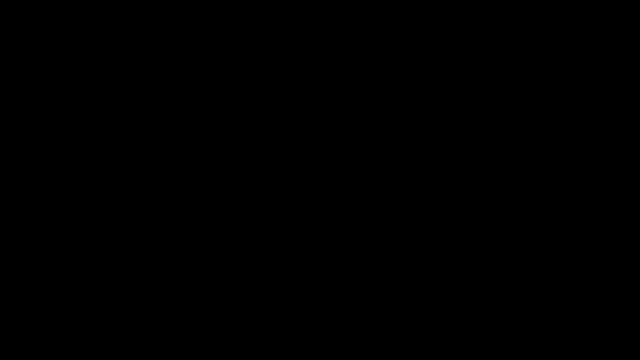 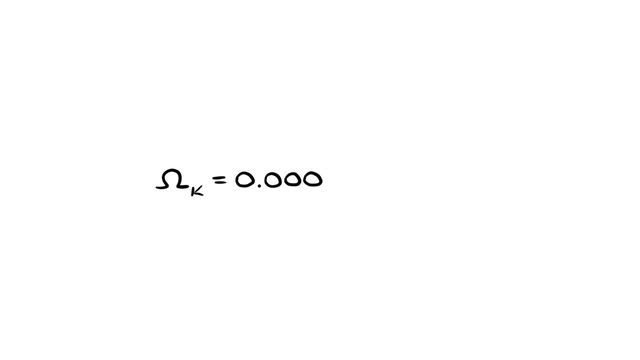 and then again in 2013 by the Planck satellite. Using the data from these experiments, along with the techniques that we just talked about, our current best measurement of the curvature of our universe is 0.0007, with a margin of error of 0.0019..